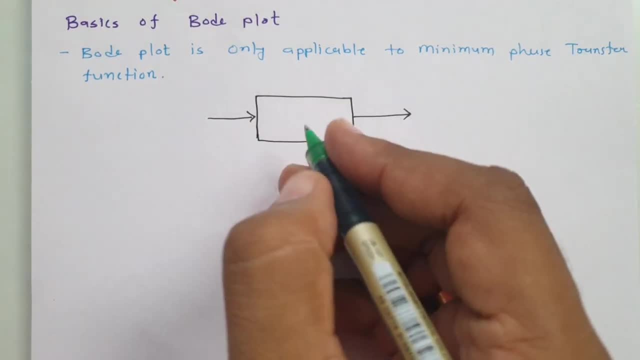 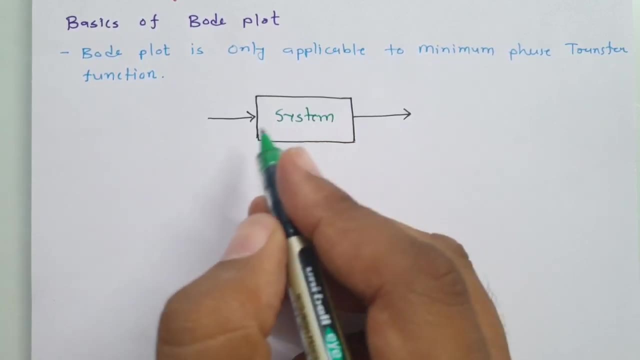 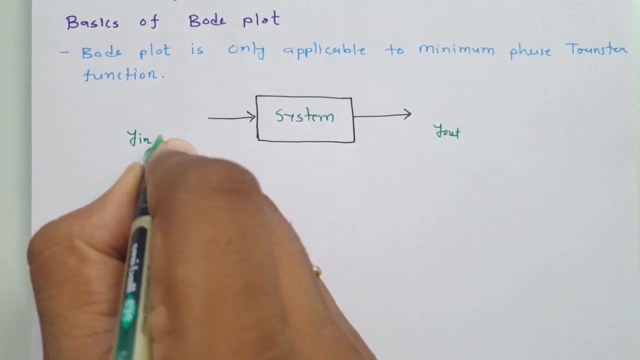 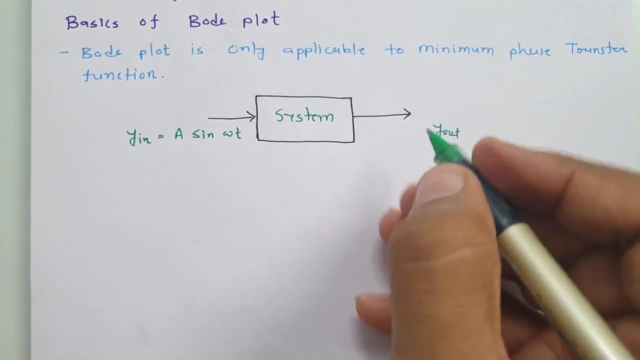 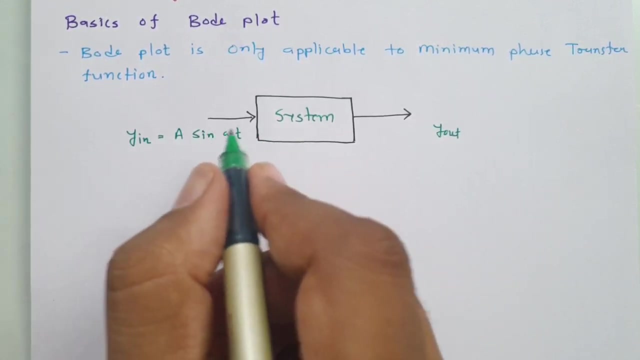 phase transfer function. now, if system is minimum phase transfer function system, in that case to plot body plot, here we give input and here we take output. if i say my input is a sine, omega t, then here we will be changing frequency, omega and we will observe two different plot. 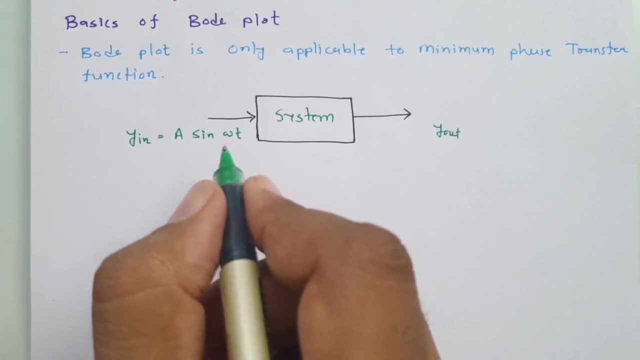 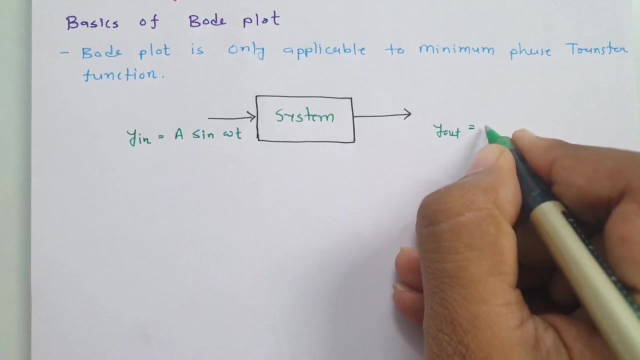 of system. one is amplitude plot and second is phase plot. amplitude plot- that is there with respect to gain of the system and phase that we are will be to observe how much change is happening. so if we change omega, then at output side there will be change in amplitude and sine omega t plus phi, where 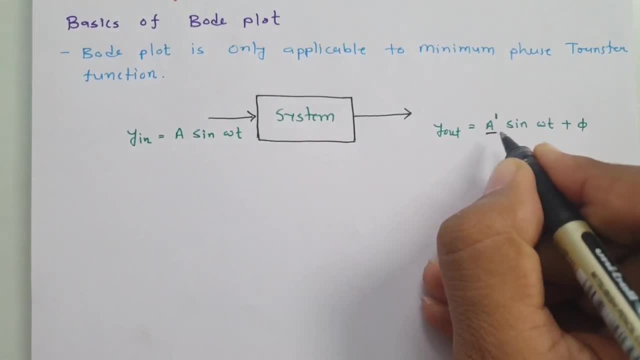 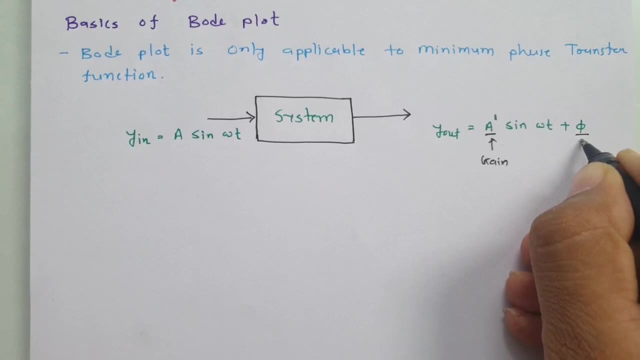 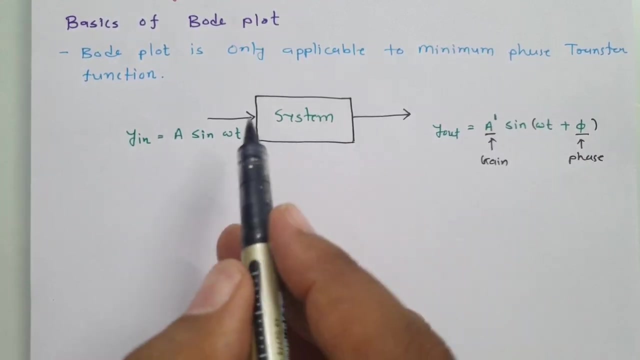 here we will be observing how much amplitude is changing. based on that, in body plot we will plot gain and by observing how much change is happening in phase, we will be plotting phase of the system, right, so here we will be varying input and we will be observing how much change is happening. 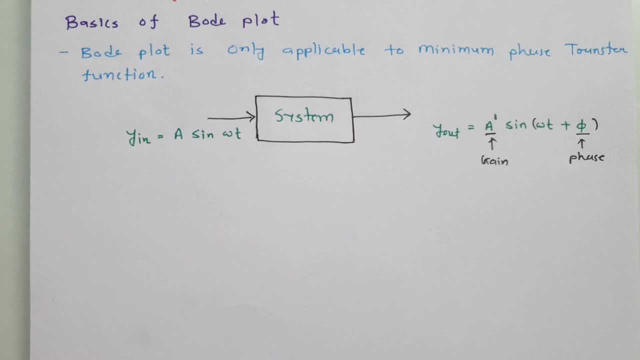 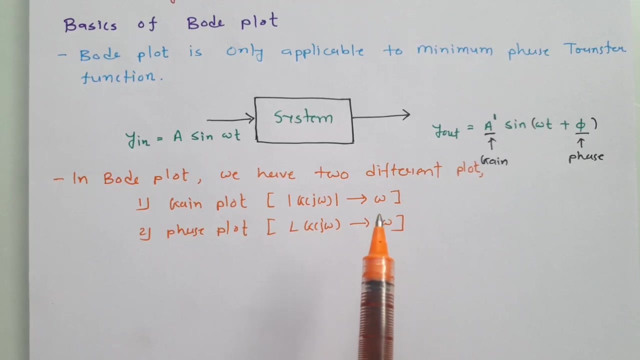 in output for body plot. in body plot there are two different plots which we are delivered to plot. one is gain plot and second is phase plot with respect to frequency. so in body plot two different plots: one is gain plot and second is phase plot. i'll show you step by step how to. 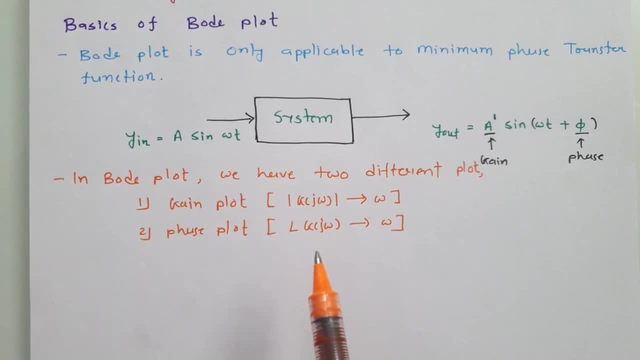 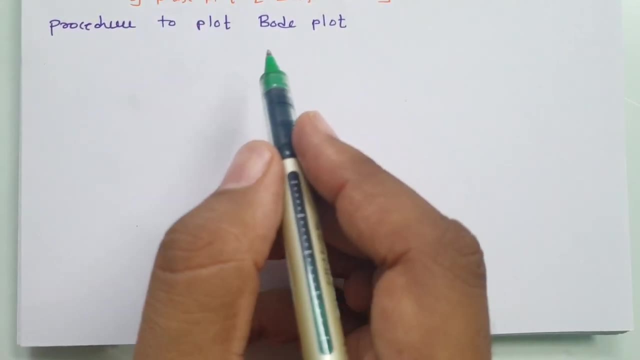 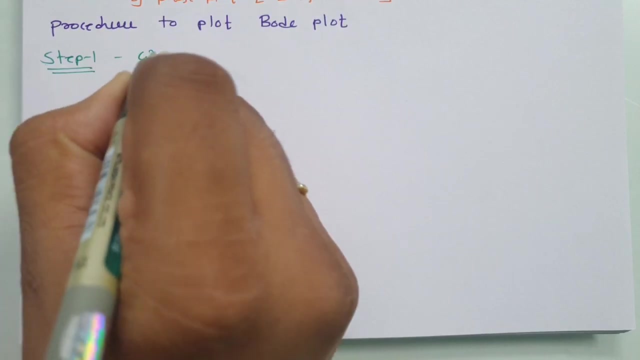 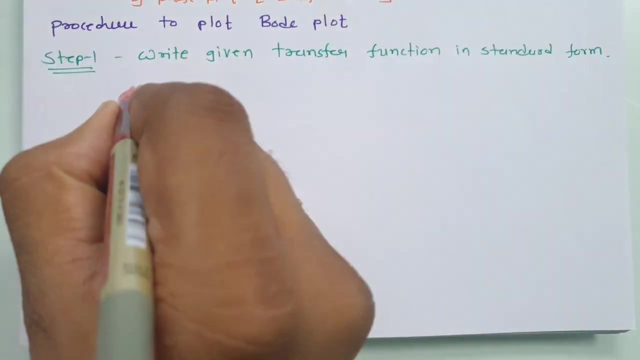 have that plotting. so now next point, that is to have a procedure to plot body plot. so when we talk about procedure to plot body plot, first step is to write given transfer function in standard form. let me explain you this by one example. so if we have been given with a system, let us say we 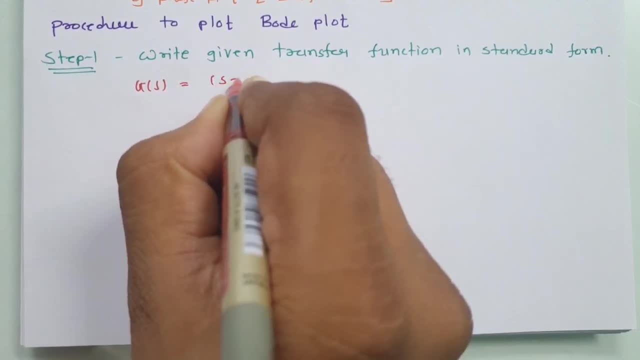 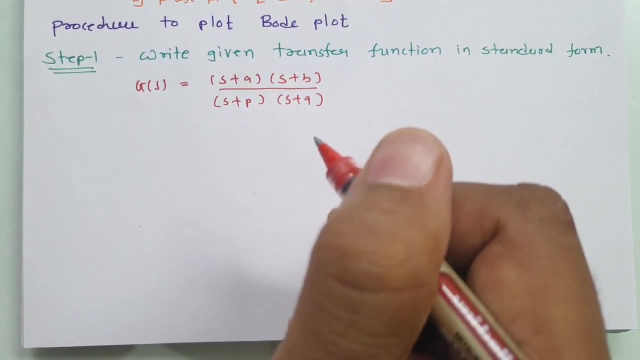 have system g of s, and that is s plus a, s plus b, divided by s plus p and s plus q. so this is what we are dealing with to write in standard form. now you can see that we have given a system g of s, and that is s plus a, s plus b, divided by s plus p. 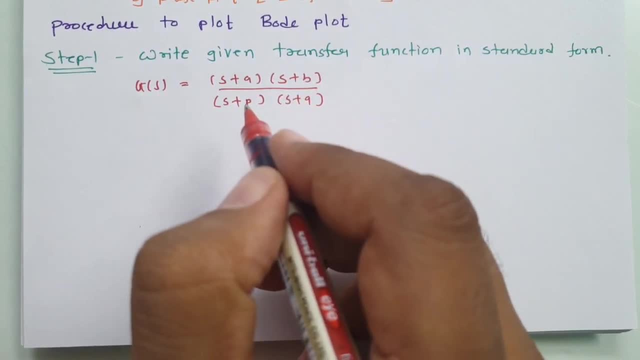 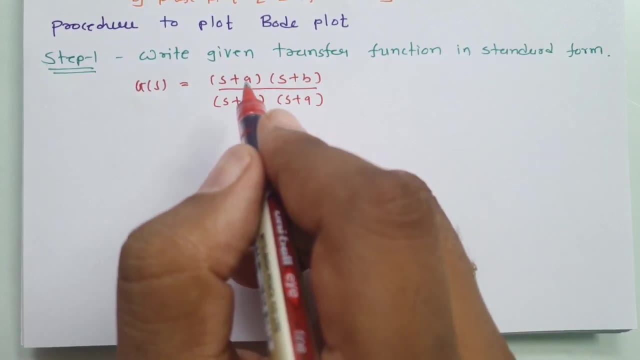 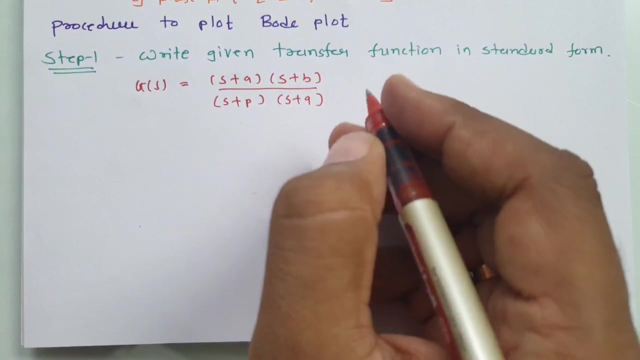 see what is standard form. standard form is like whatever poles and zeros that is there with the system. that should be written in form of one plus s divided by something. see that is what standard form. so to write this system in standard form, all we will be doing is we'll be taking a common from. 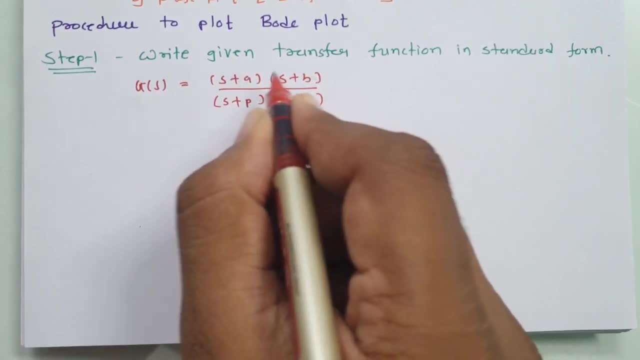 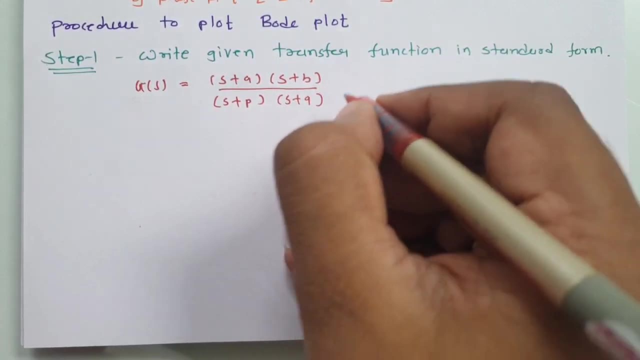 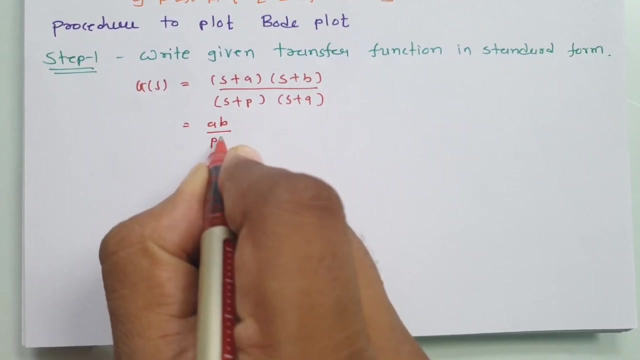 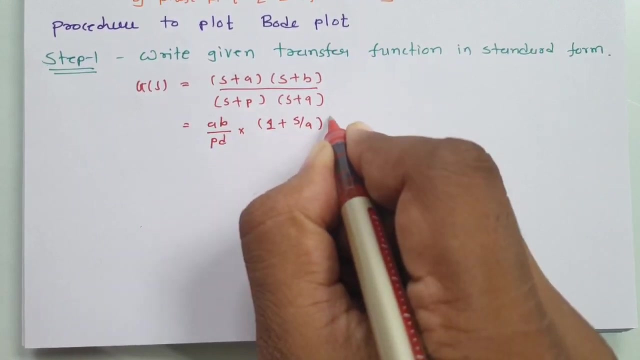 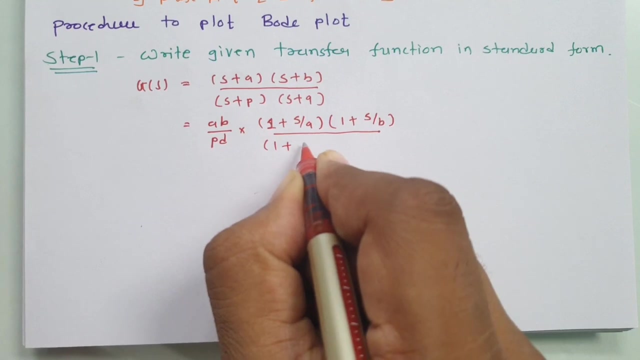 this counts b common from this, counts p common from this and q common from this. so here, if we take common like this, then here we'll be having a b divided by p, q into one plus s by a, one plus s by b, divided by one plus s by p and one plus s by q. so this is: 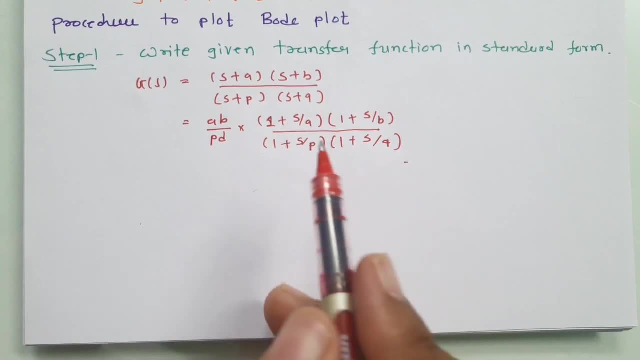 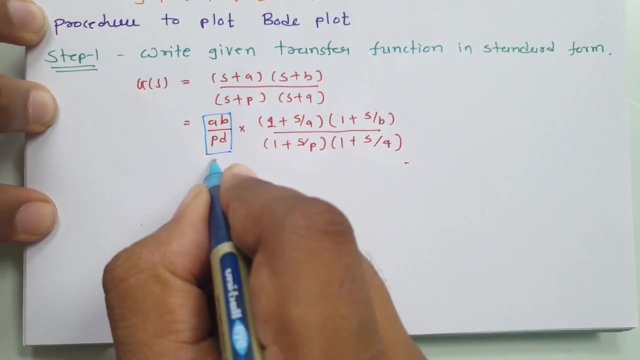 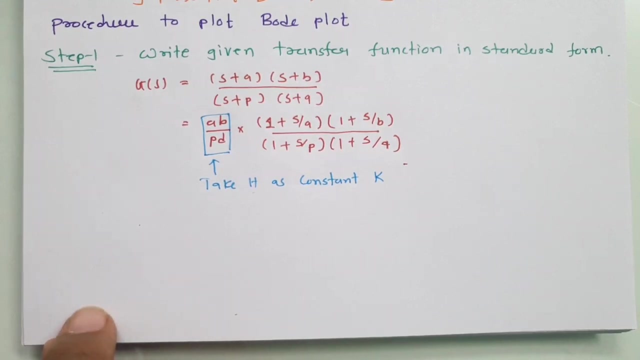 This is what standard form which we have. So first step is to write given transfer function in standard form. Now, here we have this, and that is a constant that we need to say Now. in second step, we will be identifying slope of first line for body plot. 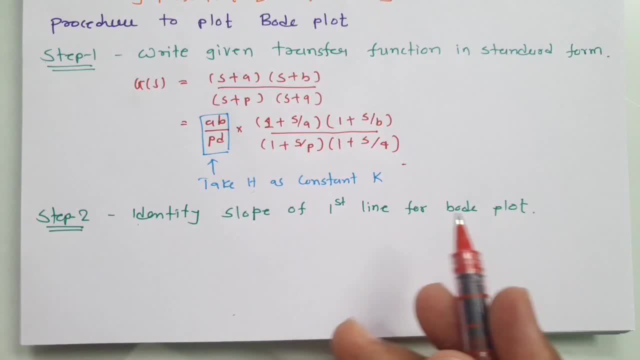 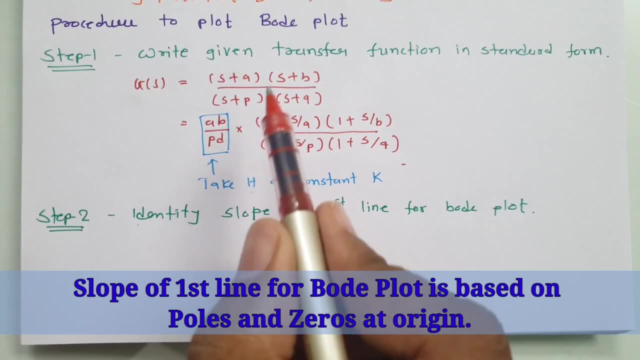 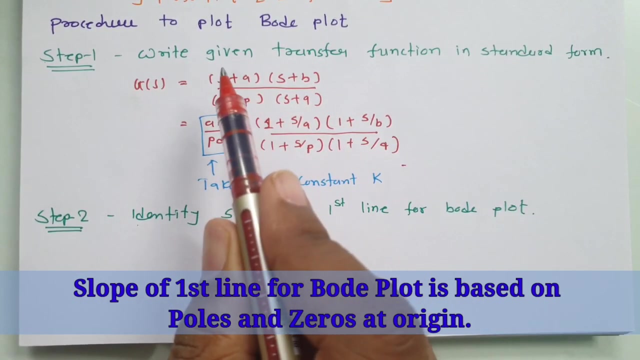 So slope of first line for body plot that is based on poles and zeros at origin. If you observe this transfer function, then in this transfer function there is no pole and zero at origin. So we can say slope of first line that will be 0 dB per decade for given system. 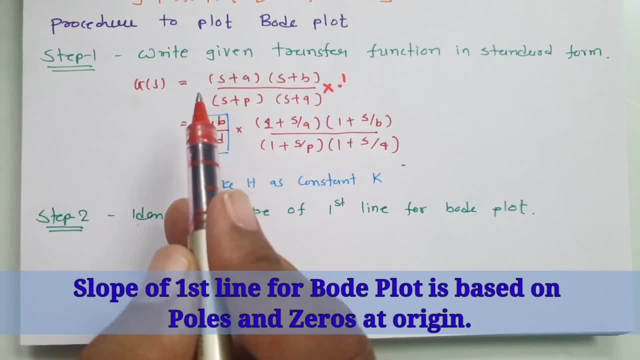 But as if I have 1. Pole at origin means this into 1 by S. In that case, slope of this system for first line that has to be minus 20 dB per decade. If this system is having two poles at origin, in that case here there will be 1 by S square. 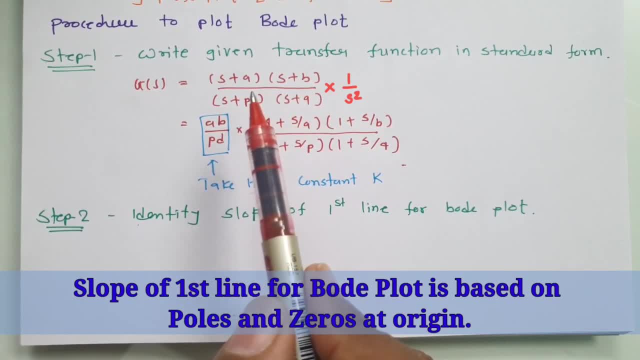 with this system Means it will be having Minus 40 dB per decade Slope of first line. Likewise, if there is 1 zero at origin, then S that we need to multiply with this system, Then slope of this system with first line that has to be plus 20 dB per decade. 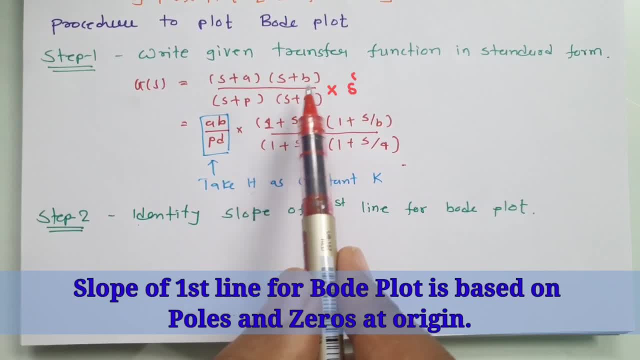 If two zeros are there at origin means multiply by S square is there with this system, Then slope of first line for this system has to be plus 30 dB per decade. So, based on poles and zeros at origin, we need to identify slope of first line. 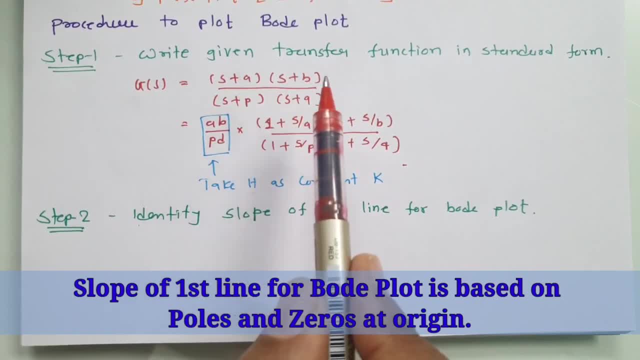 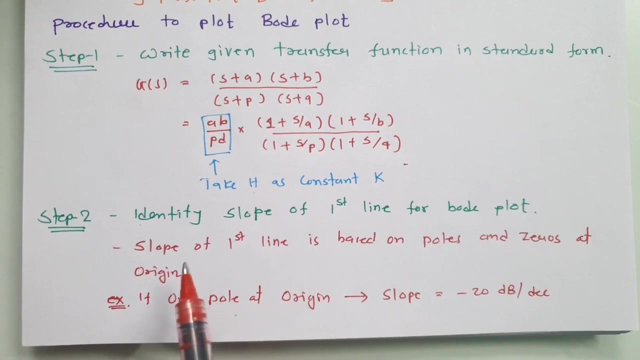 Here there is no pole and zero with origin, So we can say slope of this system will be 0 dB per decade. So slope of first line is based on poles and zeros at origin. If pole is there then slope will be minus. 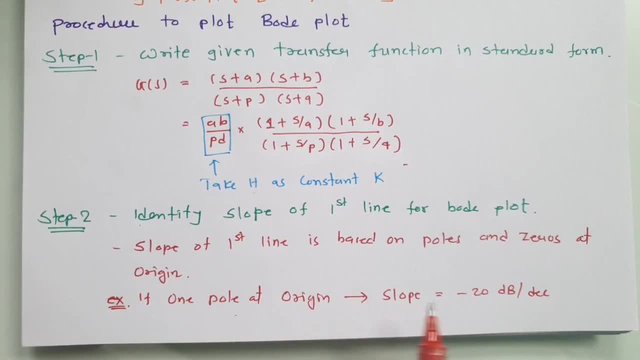 If one pole, then minus 20.. If two poles at origin, then minus 40. That is how we identify slope of first line. Now next step is to identify gain of first line at omega is equals to 1 radian per second. 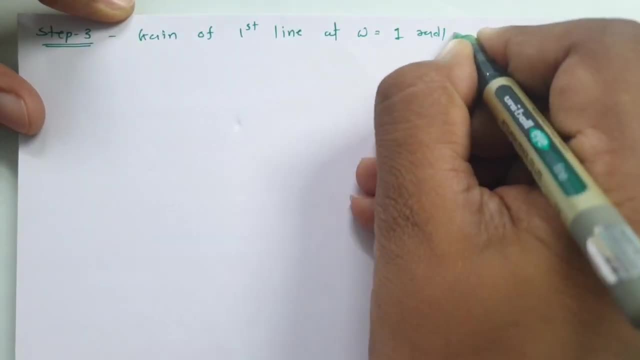 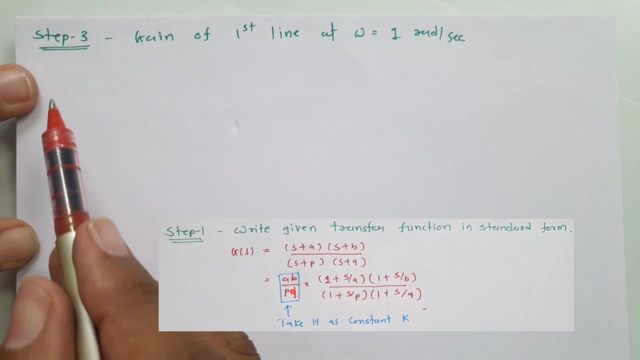 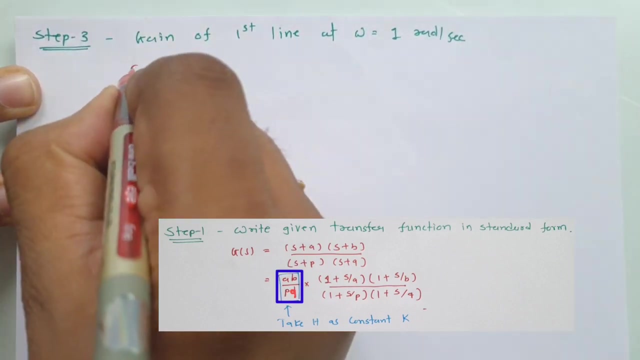 So in step 1, we have seen Standard form of transfer function in that we have identified constant k. So based on constant k, we can identify gain of first line at omega is equals to 1 radian per second And to identify gain of first line at omega is equals to 1 radian per second. 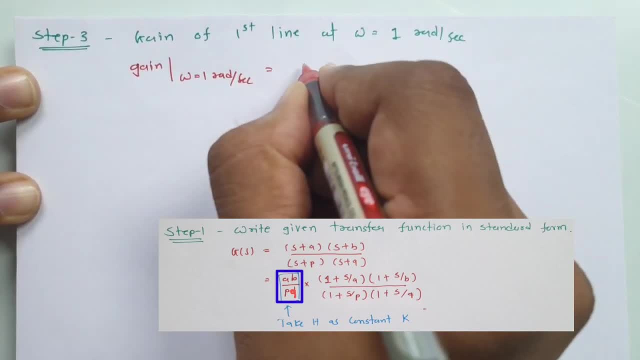 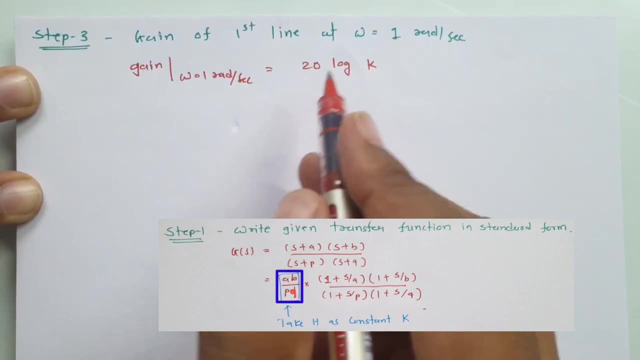 All we need to do is we just need to calculate 20 log of constant k. So this is what gain of first line at omega is equals to 1 radian per second. So now we have slope of first line and gain of first line at omega is equals to 1 radian per second. 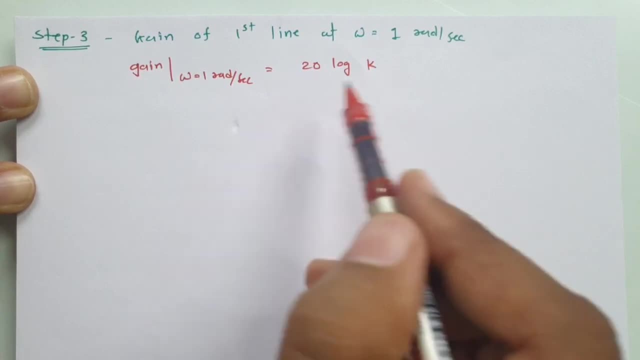 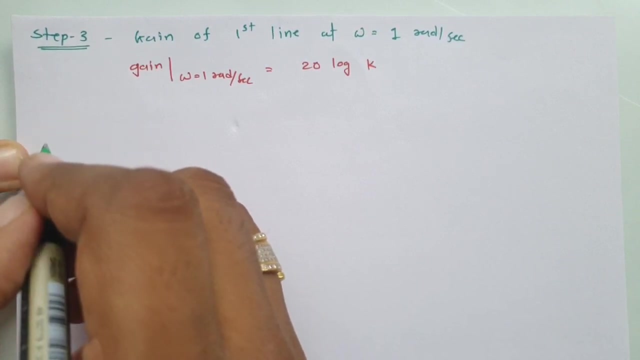 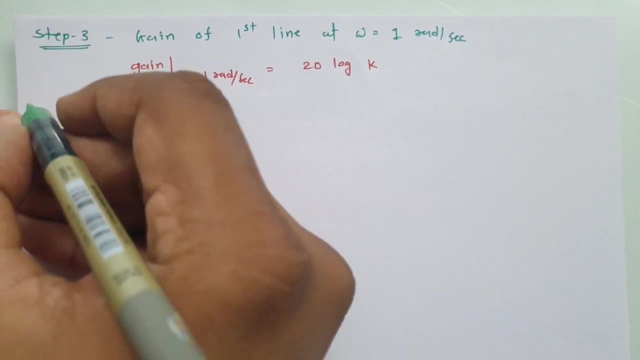 So we can start with our plotting of body plot Now. next step is to identify Slope with respect to different corner And corner frequency. So in that first we need to write All the corner frequency in ascending order And we need to identify slope of each lines. 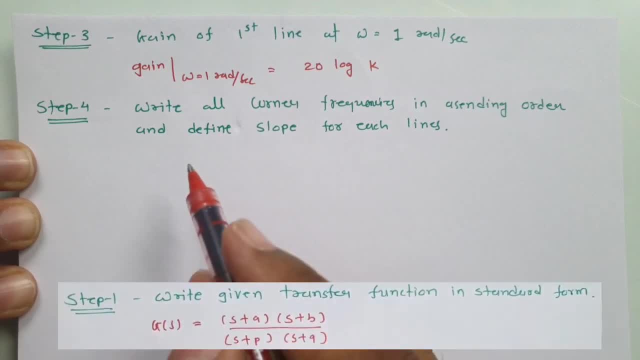 So if you observe Transfer function which is given to us, So in that transfer function you can observe There are two poles And two zeros. One zero That is there at A, Second zero is there at B. Two poles are there. 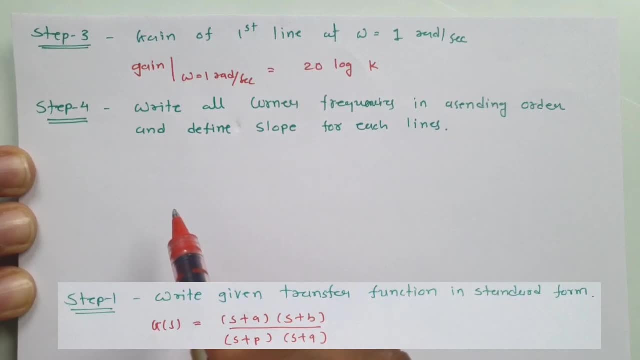 One pole is there at P And second pole is there at Q. So this frequencies are corner frequencies And we need to arrange this corner frequencies in ascending order. first, If I say I have A greater than P, Greater than B, 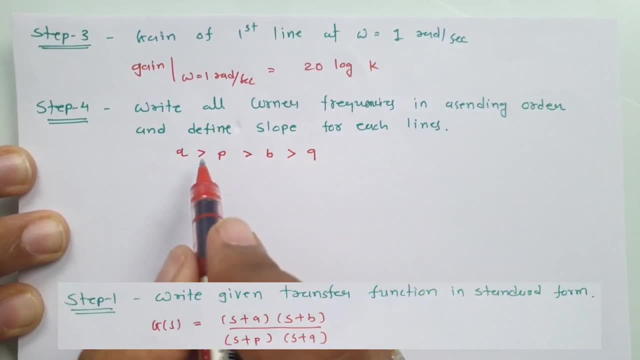 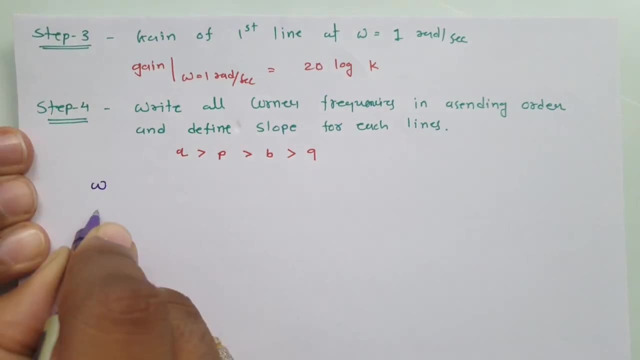 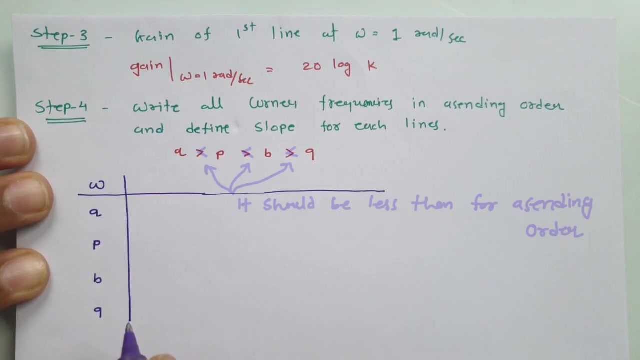 Greater than Q, Then I need to Write this corner frequency of given transfer function In ascending order. So now you can observe I have written This corner frequencies In ascending order. After that I need to mention Pole and zero. 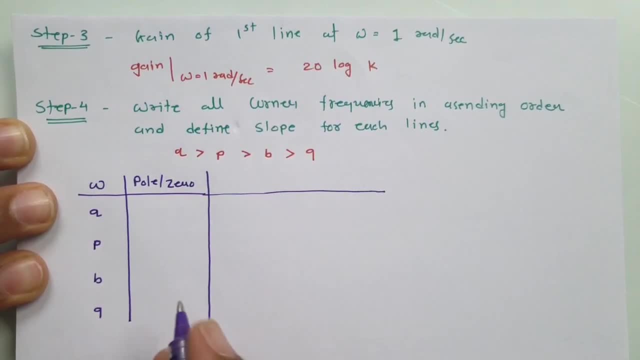 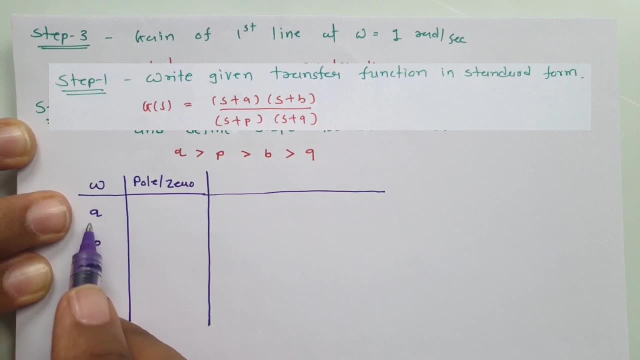 Which is there at this frequency. So you can see In transfer function: A is having Zero, P is having Pole, B is having zero And Q is having Pole, And we should know What is The slope. 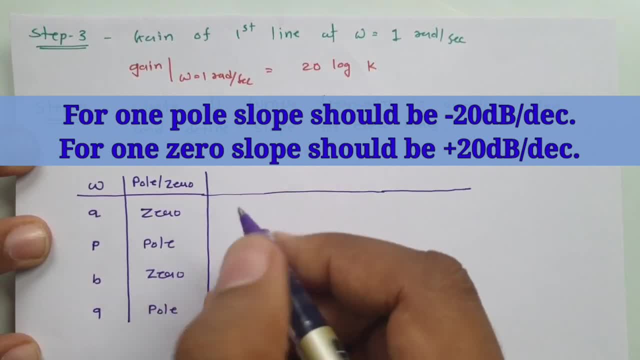 With pole and zero. If you have a pole, In that case Slope Has to be Minus 20 dB per decade, And if you have Zero, In that case Slope has to be Plus 20 dB per decade. 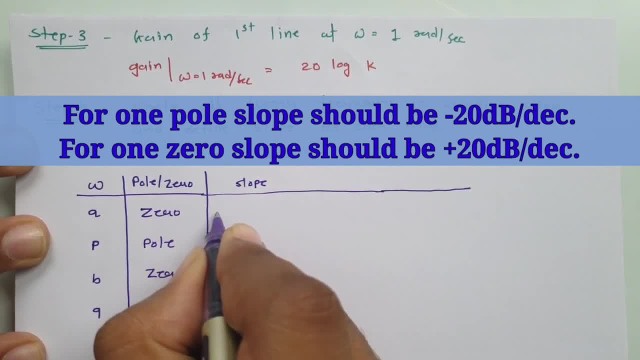 So here zero is having slope That is Plus 20 dB per decade. Here pole is having slope That is Minus 20 dB per decade. Here zero is having slope That is Plus 20 dB per decade. 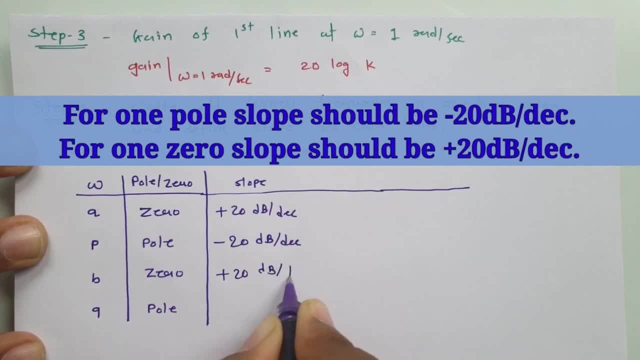 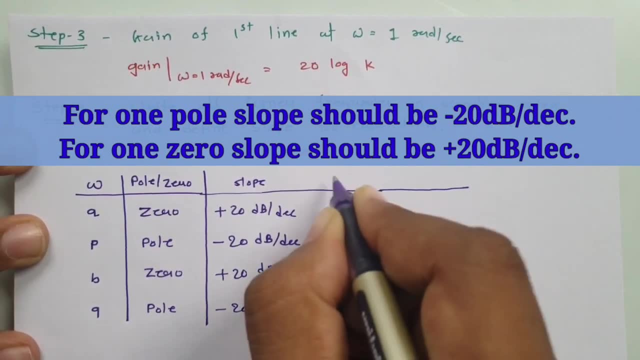 And here Pole is having slope That is Minus 20 dB per Decade And At last We will have to identify Resultant slope. Now, in resultant slope, First line That is Having Corner frequencies. 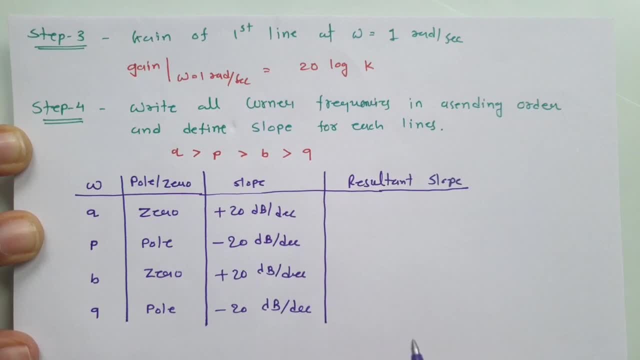 In ascending order And Zero Is having Slope That is Plus 20 dB per decade. So here For first line Resultant slope Will be 20. dB Per Decade. Now 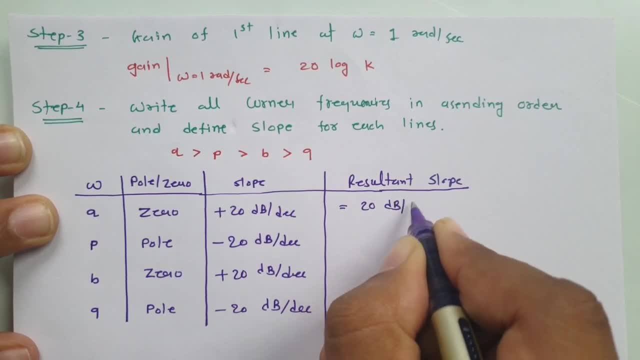 After second corner frequency. You see There is a pole. So this slope Plus Previous slope That we need to do, So 20. Minus 20. So here Zero Slope Will be there And 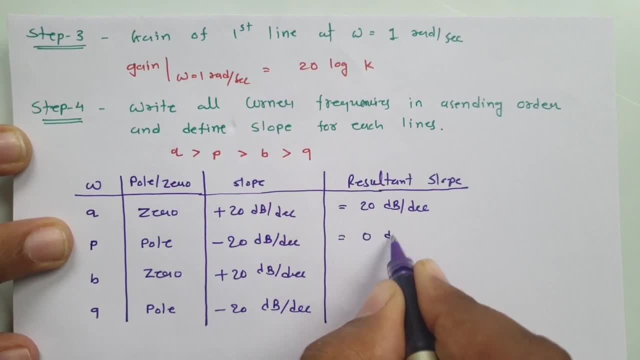 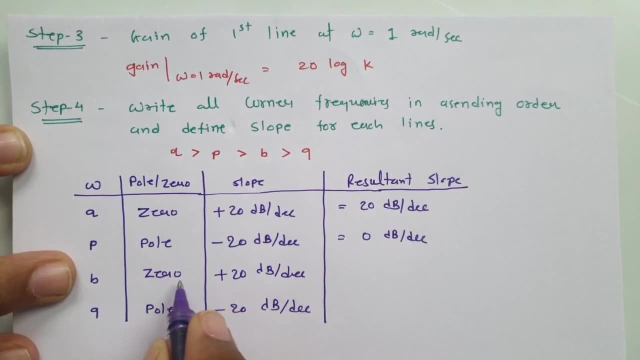 Here Zero Slope Is having 20. dB Per Decade. Now This slope Plus Existing slope, With this Corner frequency Which is B, So Zero Plus 20.. So that is. 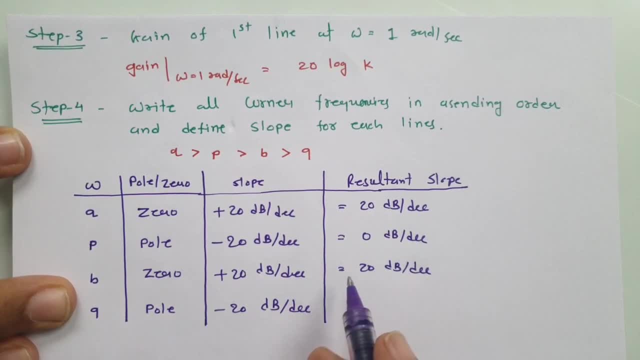 Plus 20. dB Per Decade And With Last Corner frequency, Which is Q. So that is Having Slope. And In Next Video I'll Explain You This. 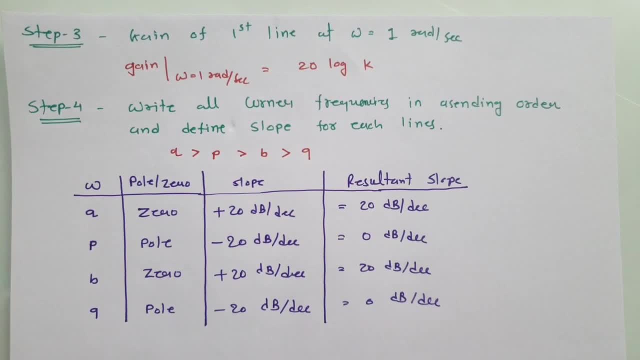 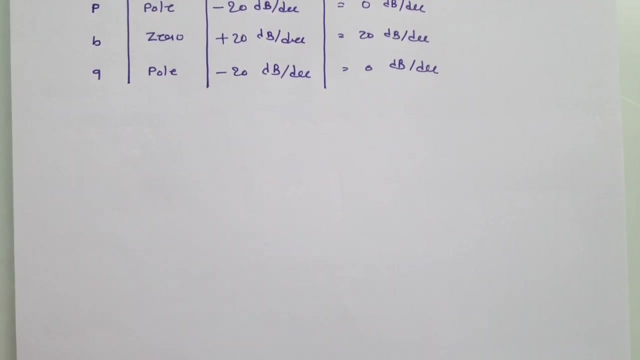 By Practical Example, So that Will Be More Clear. Here You Just Understand How Procedure Is There. Now Next Step Is: So Let Us Try To. 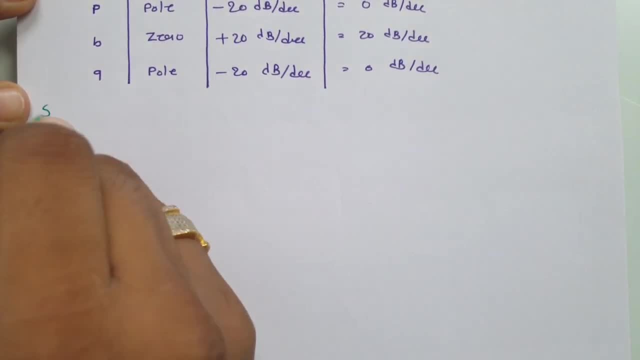 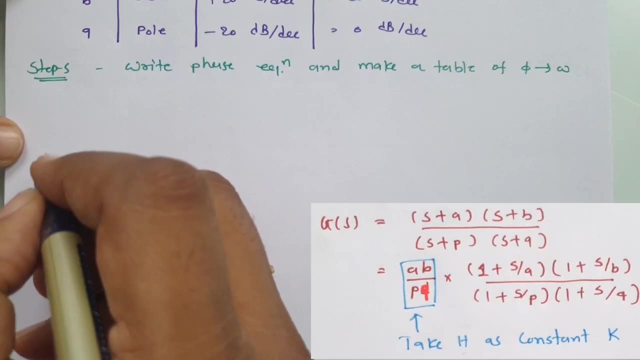 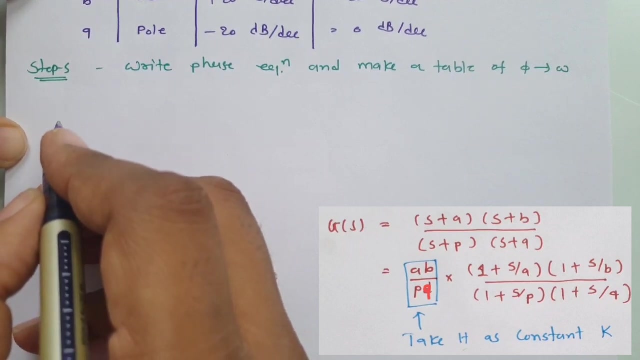 Understand How To Write Phase Function And How To Make A Table Of Phase With Respect To Frequency. So If You Observe, Here We Have 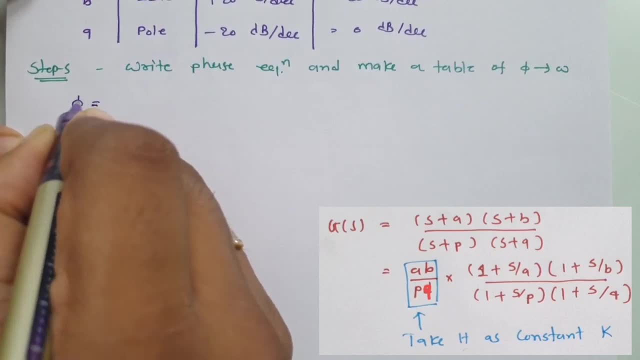 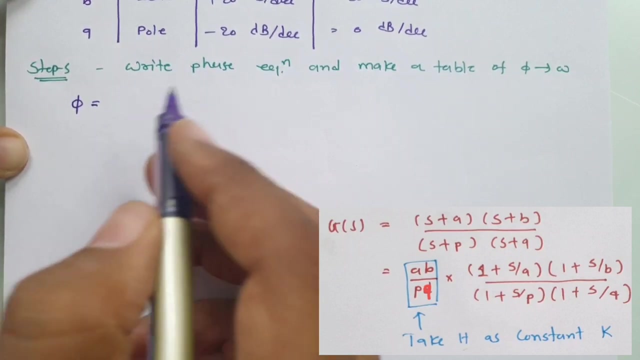 This Function, Then In This System We Need To Place S Is Equals To J, Omega Right, And If You Place S Is Equals To J, 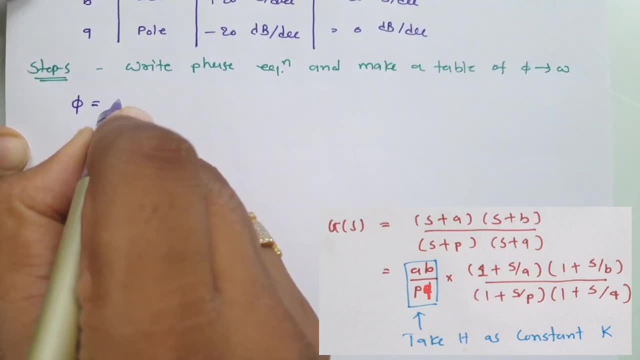 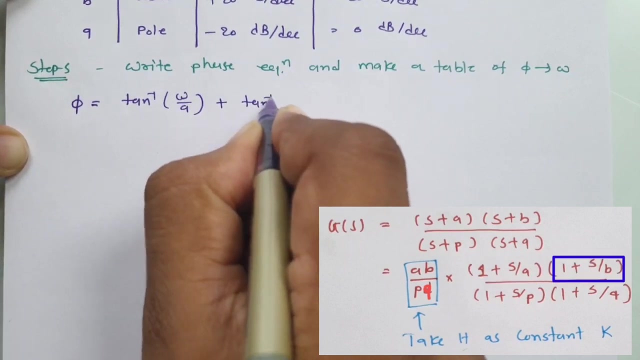 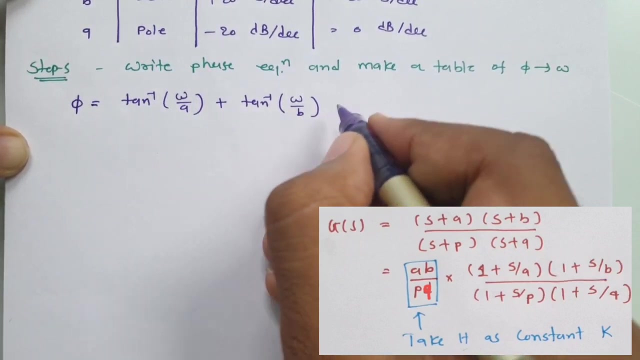 Omega There Is A Phase Is Negative And For Pole At P Phase Is Tan Inverse Omega By A And That Is Positive Plus For. 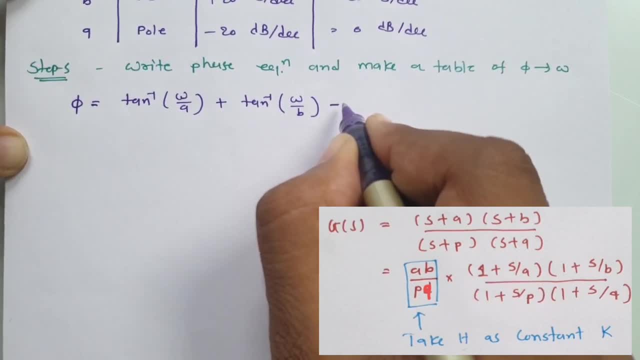 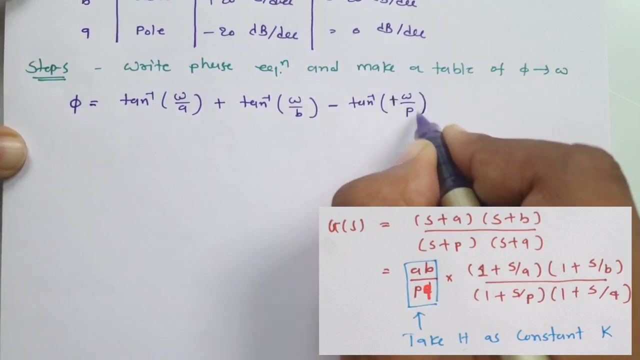 Second Zero At B Phase Is Tan Inverse Minus Omega By P, Here Already Minus That I Have Took It Outside, So I Need. 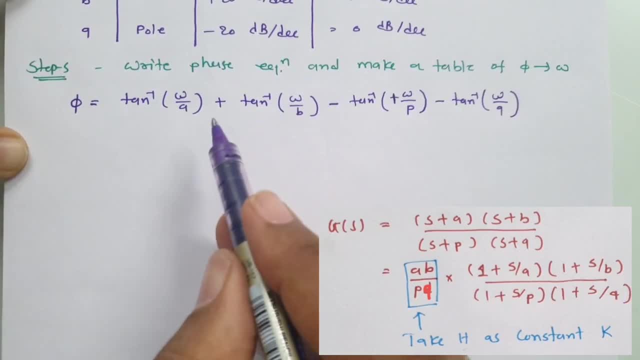 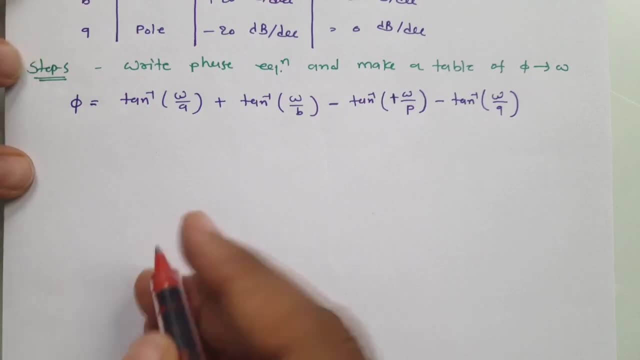 To Write Plus Over Here: Minus Tan. Inverse For Second Pole Phase Is At P Phase. Is At P Phase, Is Minus Omega And. 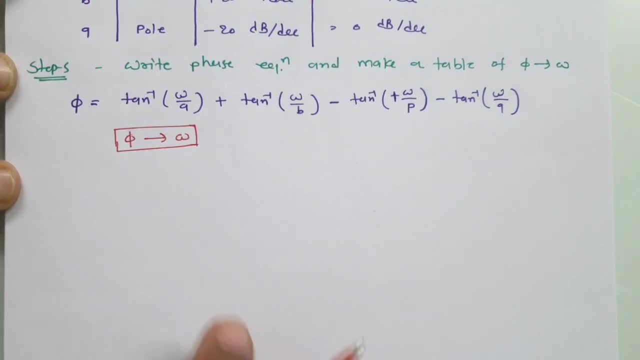 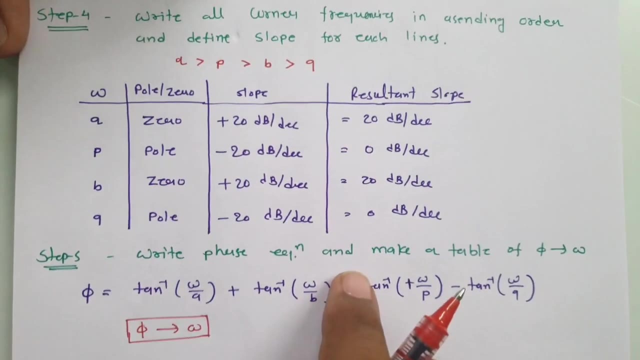 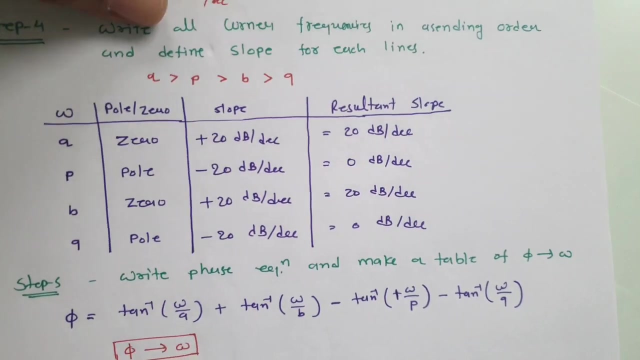 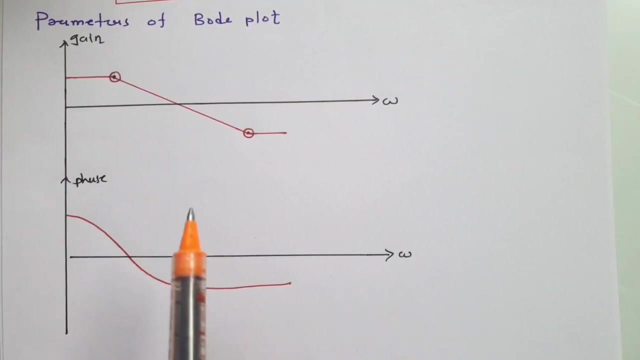 I Can Make A Table Of Phase With Respect To Frequency By Writing Different Values Of Phase. Next I'll Be Explaining Different Parameters Of Body. 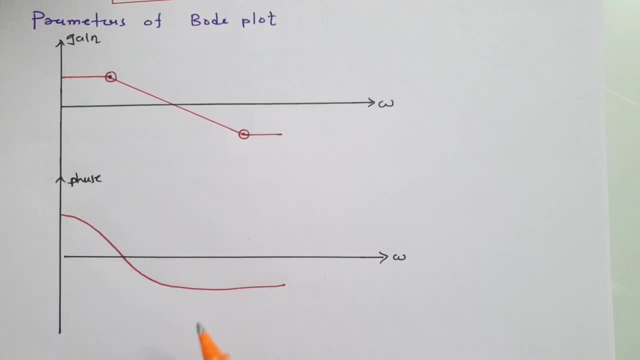 Plot. So Here We Have Been Given, With One Body Plot Right, And In This Body Plot We Have Gain. And Here, In Phase We Need, 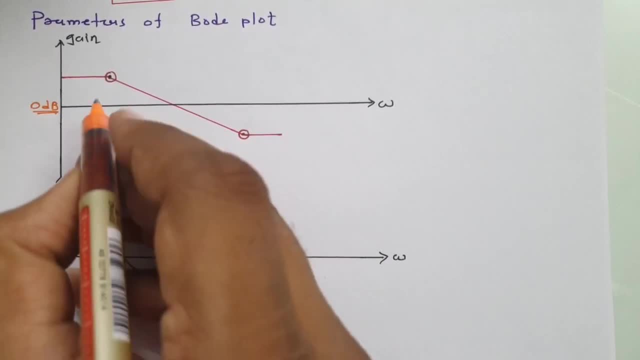 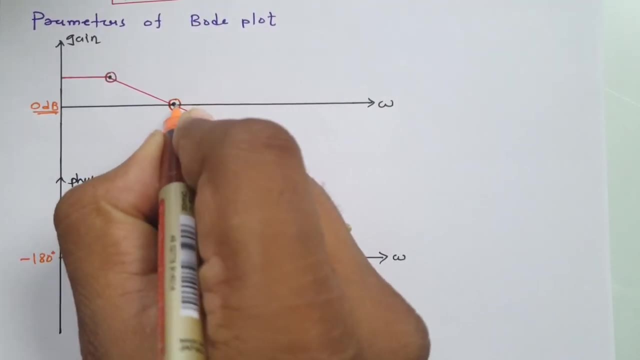 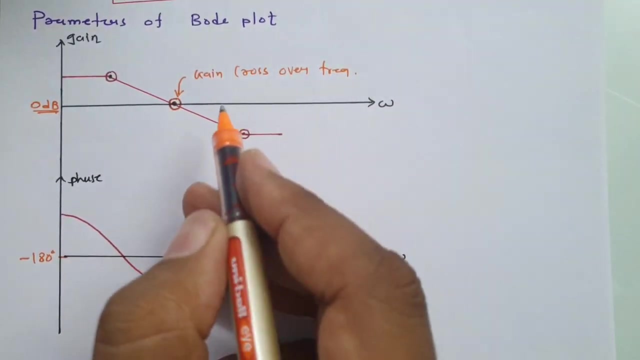 To See Minus 180.. Degree Phase: Right, So In 0 dB Line. If You Observe This Gain Plot That Is Intersecting Over Here. 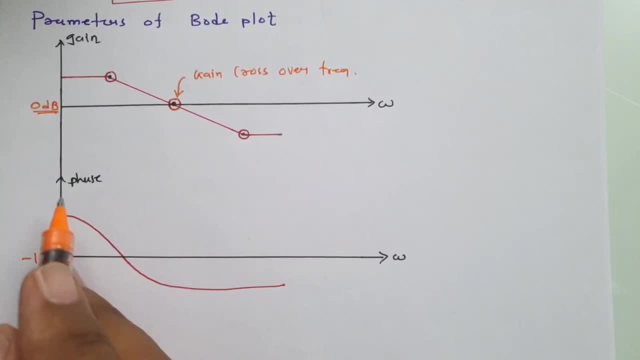 So This Point: If You See This Phase Plot, Then Phase Is Intersecting Here At Minus 180. Degree. So This Is Referred As 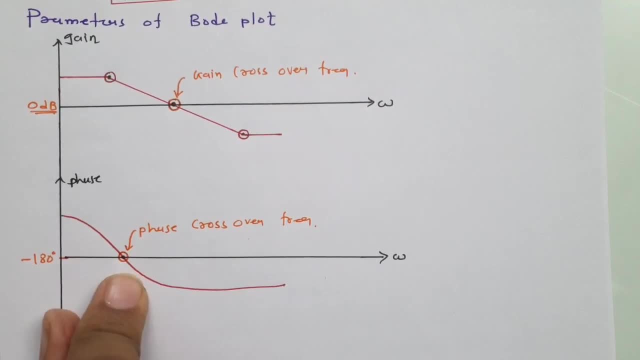 Phase Cross Over Frequency. So Phase Cross Over Frequency Is Once We Have Gain Cross Over Frequency And Phase Cross Over Frequency, We Need To Extend. 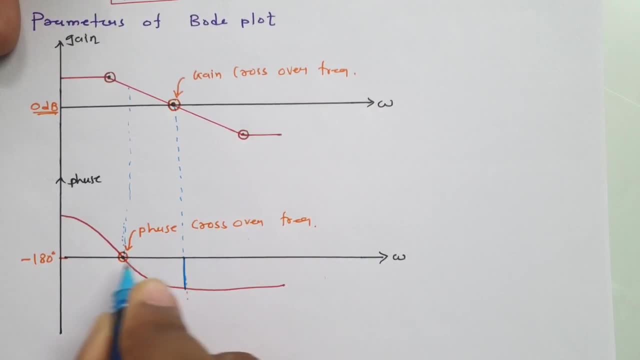 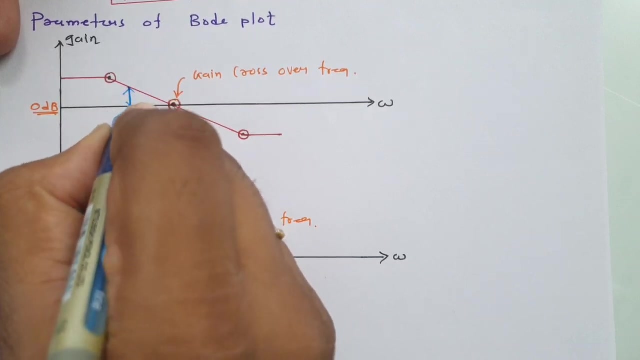 This Line On Each Other. Now, Once We Have Extended This Line, We Extend This Line Over Gain, Then This Is The Margin Of Gain, This 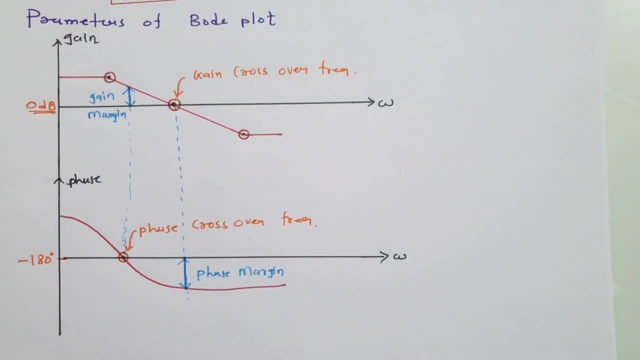 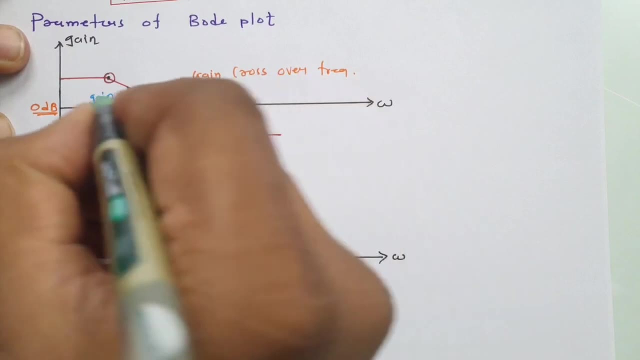 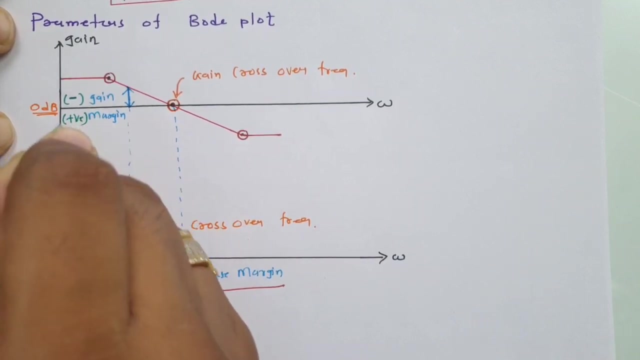 Is The Margin Of Gain With Respect To 0. Db And That Is Referred As Gain Margin That Is Negative Below 0. Db, And 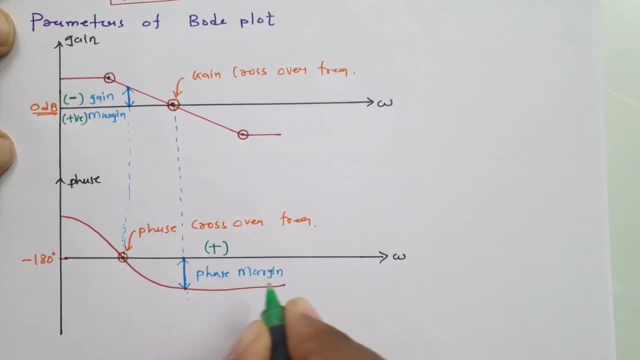 Phase Margin That Is Positive Above Minus 180.. And That Is Negative Below Minus 180.. Right, So This Is How Gain Margin Stability Is. 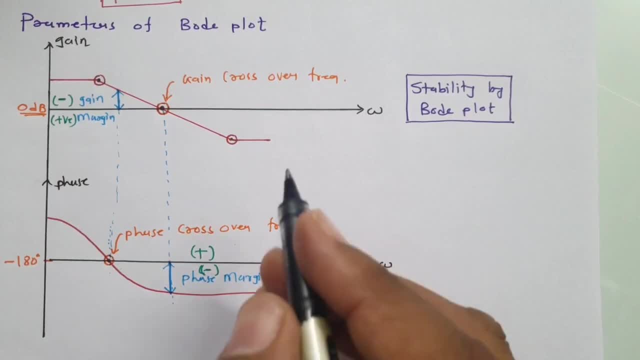 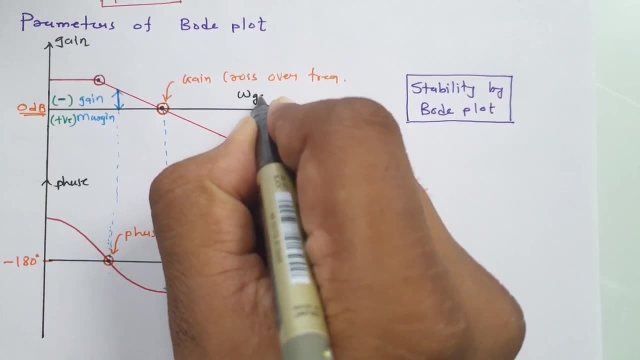 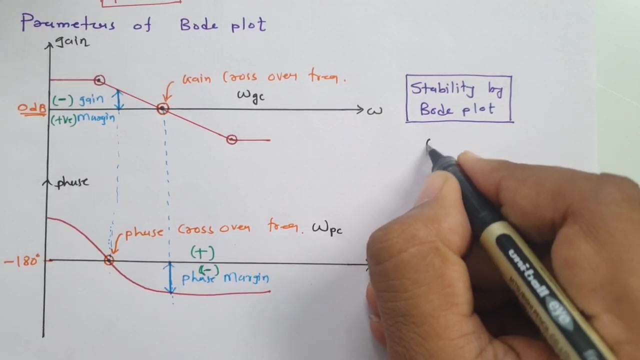 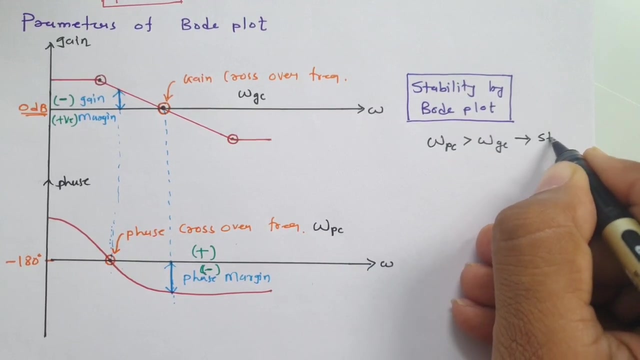 There With Border Plot. So Stability Of Border Plot That We Can Identify By Gain Cross Over Frequency And Phase Cross Over Frequency. Gain Cross Over.